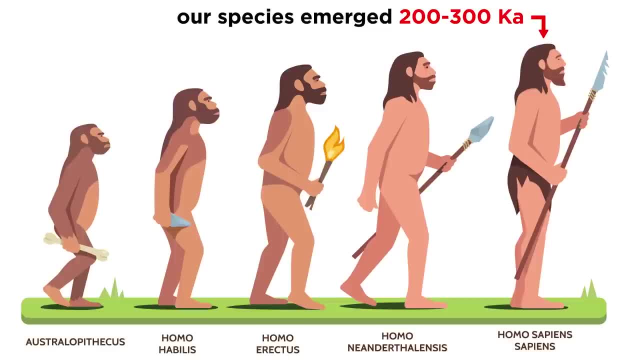 or humans, emerged between 200,000 and 300,000 years ago in Africa, But this fascinating story will have to be saved for the upcoming Anthropology series. By the Cenozoic era, most of Earth's continents were near their current locations, except. 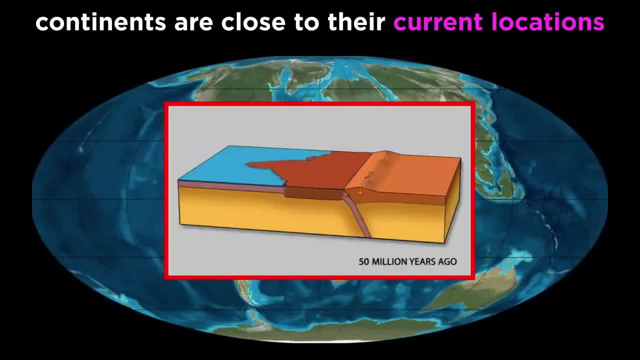 for India. The Indian continent was making a beeline toward Asia during the early Cenozoic, with collision and orogeny occurring around 50 million years ago. This event initiated uplift of the Himalayan mountains and is still occurring to this day. Additional, smaller 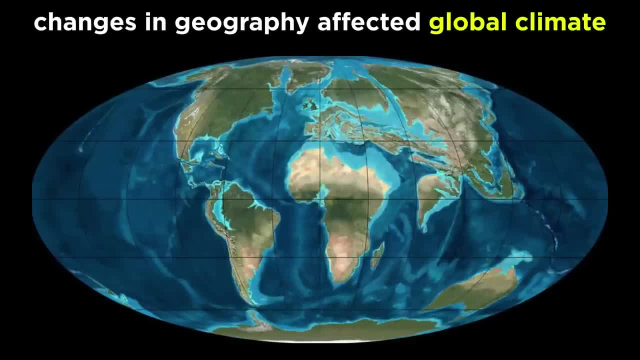 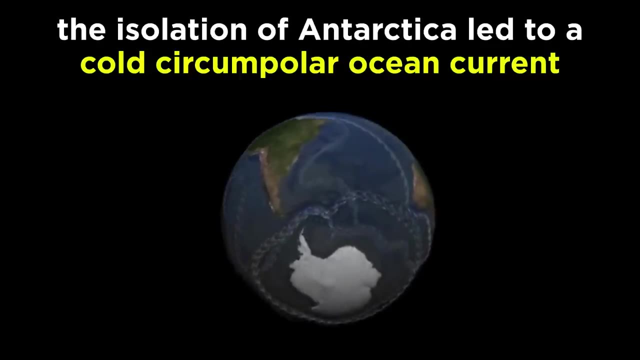 changes in geography greatly impacted the Cenozoic climate, For example. Antarctica became an isolated continent around 34 million years ago as Australia and South America broke away, moving northward. This led to the development of a cold ocean current around Antarctica. 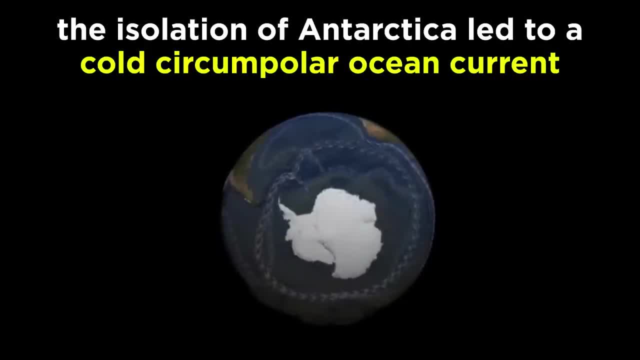 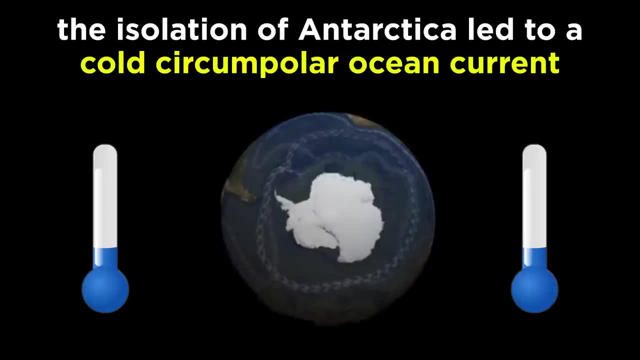 helping trap colder air over the continent. The development of the so-called circumpolar current led to global cooling and the development of the first permanent Antarctic ice shield. This is the first time in centuries that a cold ocean current has been trapped in the 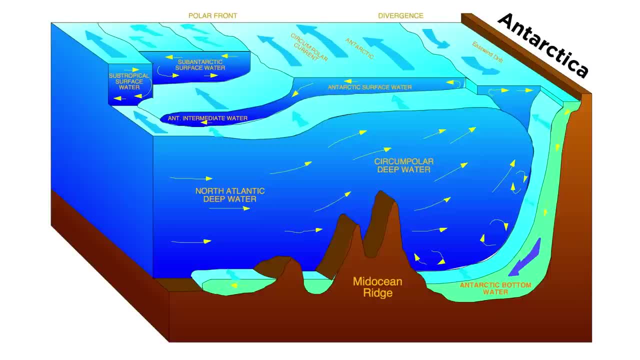 sheet marking the beginning of the modern ice age. The global cooling was caused by the development of a robust oceanic circulation where the cold, dense water of the circumpolar current sinks down and spreads out. This led to the cooling of the lower ocean, which set the stage for more atmospheric CO2. 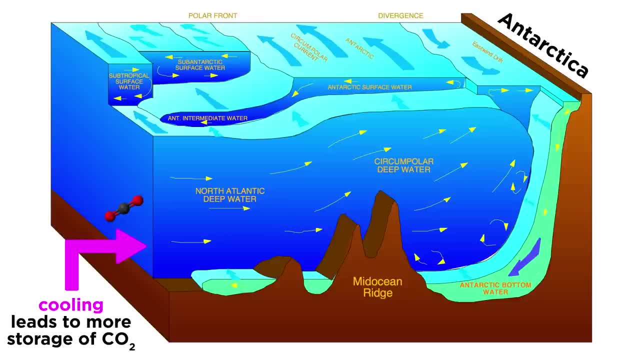 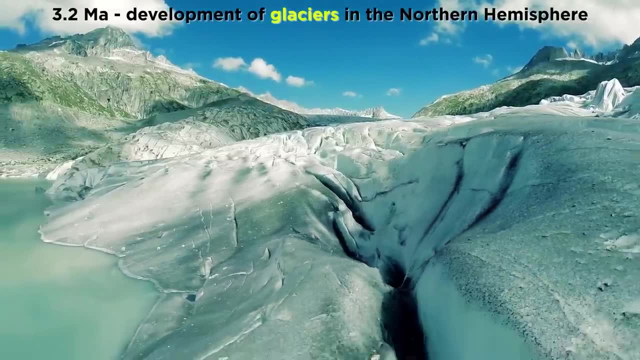 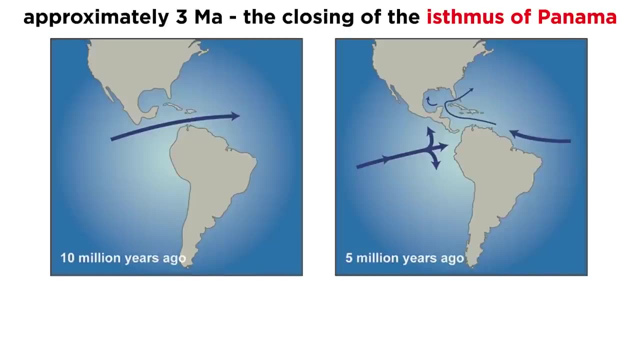 to be stored as sediment on the ocean floor, reducing greenhouse warming. The next major change was the development of glaciers in the Northern Hemisphere, which existed by around 3.2 million years ago. The cause of this is still debated, but it was probably related to the closing of the. 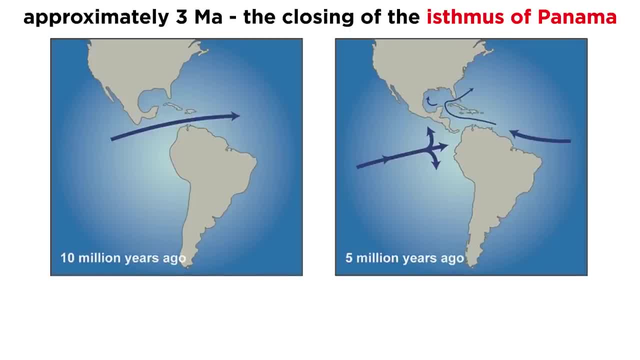 Isthmus of Panama, which occurred around the same time. The Pacific and Atlantic Oceans used to be connected where Panama is today, which allowed their waters to mix. Since the closing of the Isthmus, the Atlantic Ocean has become much saltier, which initially 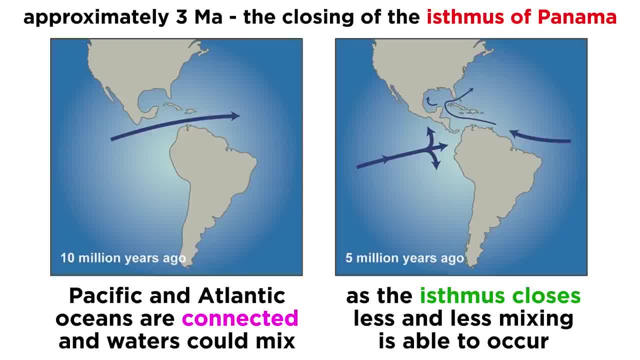 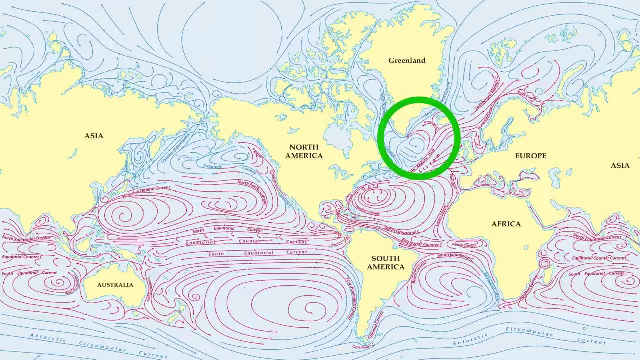 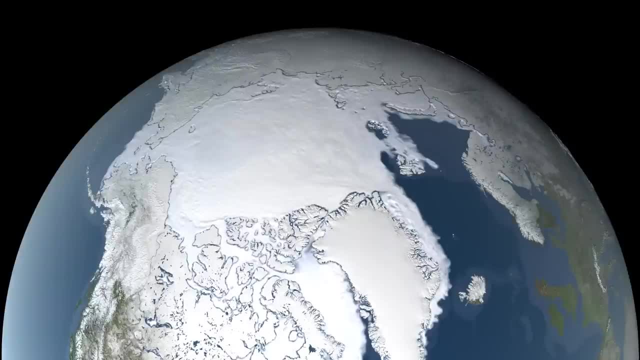 initiated a reorganization of ocean circulation. Gulf stream waters stopped circulating through the Arctic Ocean, instead sinking to the sea floor around Greenland and spreading out. This shut off the transport of warm water to the Arctic Ocean, causing the surrounding regions of Greenland, Canada and Northern Europe to cool and develop permanent ice sheets.